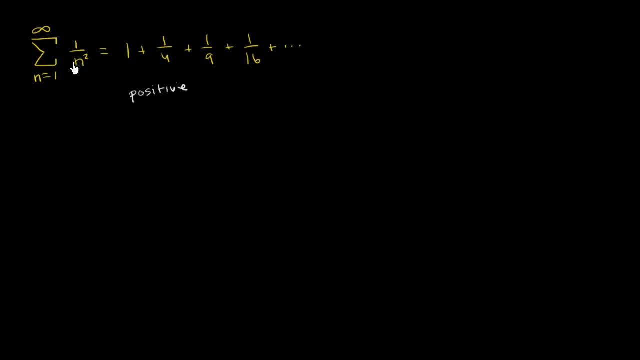 And because they're all positive, we know that this sum right over here, if it does converge, is going to be greater than zero. So the only reason why it wouldn't converge is if somehow it goes unbounded towards infinity, which we know. if this was one over n. 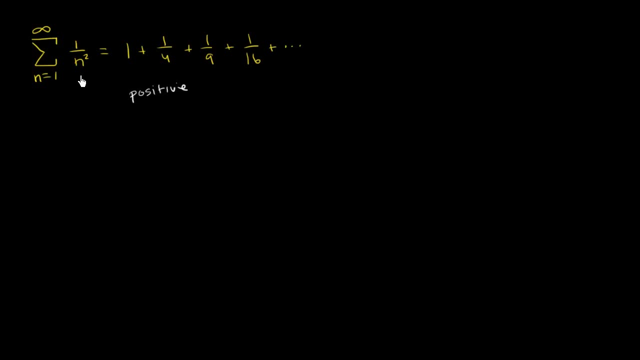 it would be unbounded towards infinity. So this has- that's a possibility here. So if we could show that this is bounded, then that will be a pretty good argument for why this thing right over here converges, Because the only reason why you could diverge- 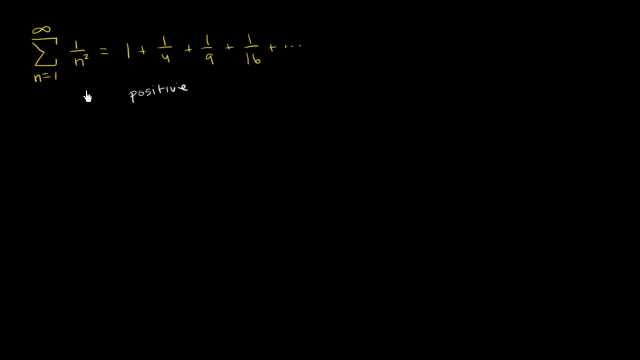 is if you went to either positive infinity or negative infinity. We already know that this thing isn't going to go to negative infinity because it's all positive terms, or you could diverge if this thing oscillates, But it's not going to oscillate because all of these terms. 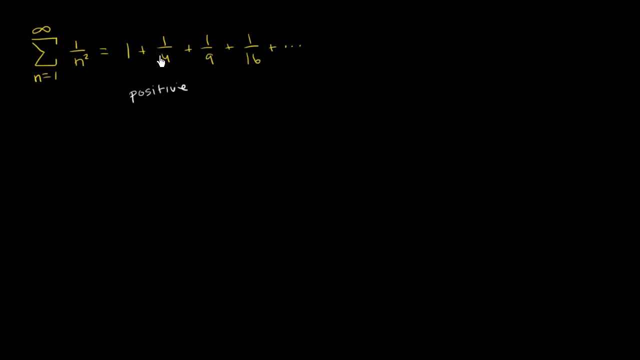 are just adding to the sum, None of them are taking away, because none of these terms are negative. So let's see if we can make a good argument for why this sum right over here is bounded, And especially if we can come up with the bound. 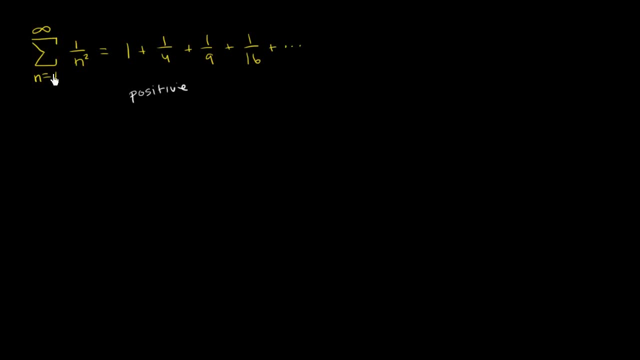 then that's a pretty good argument for that. this infinite series should converge, And the way that we're gonna do that is we're gonna explore a related function. So what I wanna do is I wanna explore f of x is equal to one over x squared. 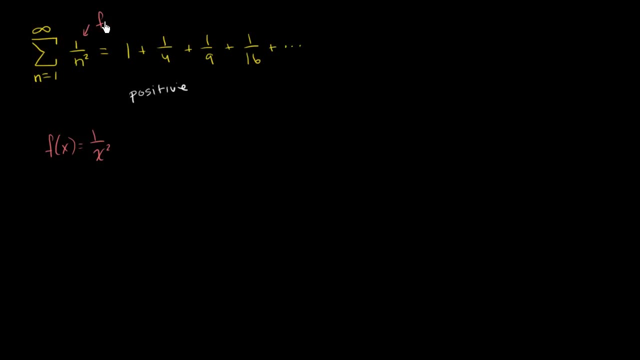 You could really view this right over here: one over n, squared as f of n, if I were to write it this way. So why is this interesting? Well, let's graph it. Let's graph it. So that's, the graph of y is equal to f of x. 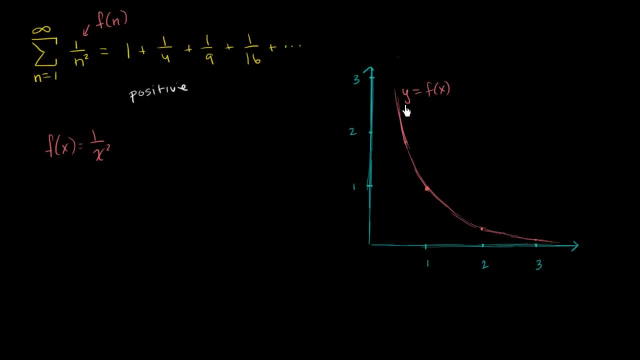 Y is equal to f of x. And notice, this is a continuous positive decreasing function, Especially over the interval that I've, or over the interval that I care about right over here, I guess we could say over the for positive values of x. 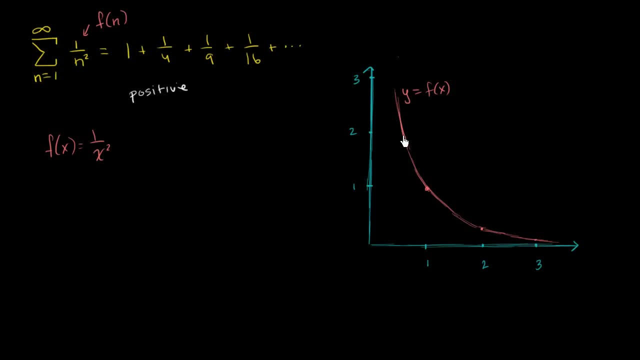 it is a continuous. it is a continuous positive decreasing function, And what's interesting is we can use this as really an underestimate for this area right over here. What do I mean by that? Well, one, this first term, right over here. 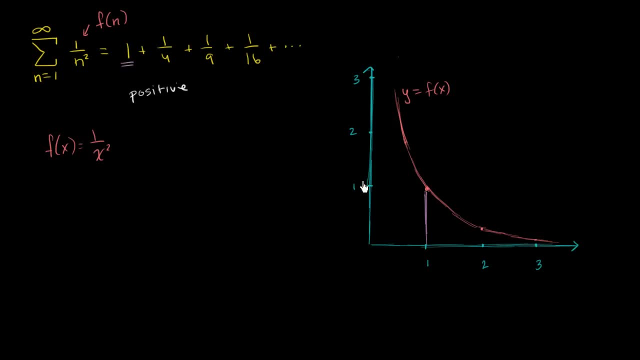 you could view that as the area of this block right over here. That is f of n, or I guess you could say f of one high and one wide, So it's going to be one times one over one squared, or one This term. let me make sure I'm using different colors. 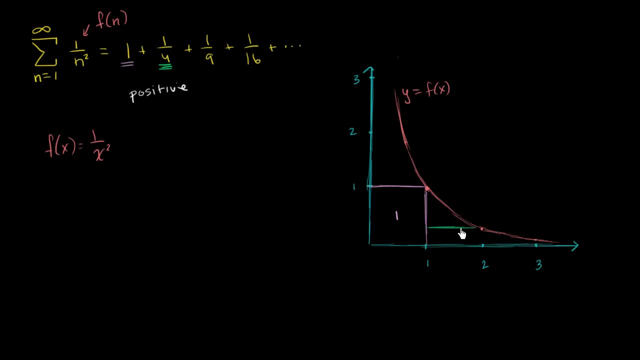 This term right over here. that could represent the area of this block, which is one fourth high and one wide. So it is going to be, it's going to have an area of one fourth. What could this one represent? Well, the area of the next block. 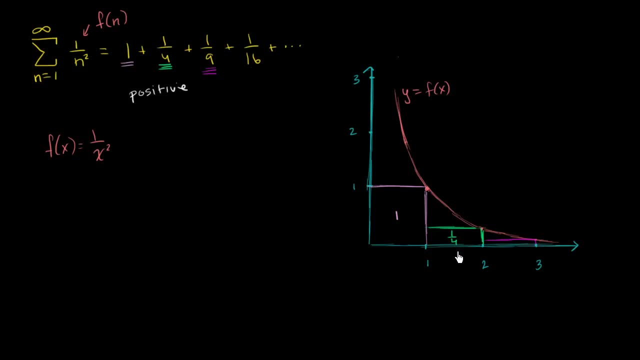 if we're trying to estimate the area under the curve- And this might look familiar from when we first got exposed to the integral, or even before we got exposed to the integral, when we were taking Riemann sums. So that right over here, 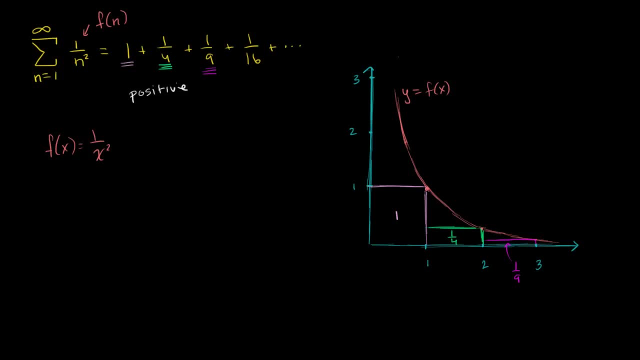 that area is going to be equal to one ninth, So what's intriguing about this is we know how to find the exact area, especially, or the exact area from one to infinity- from x equals one to infinity, So maybe we can use that somehow. 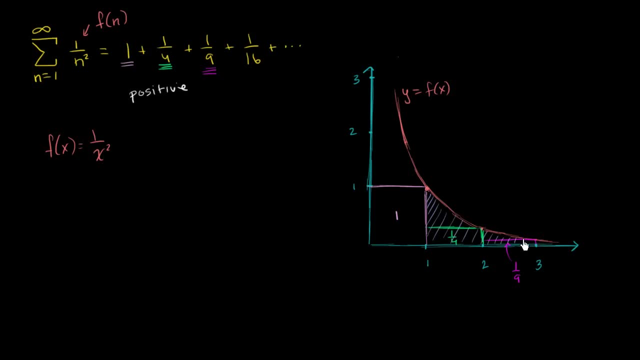 We know what this area is right over here, which we can denote as the improper integral from one to infinity of f, of x, dx. We know what that is and I'll figure it out in a little bit. And if we know what this is, 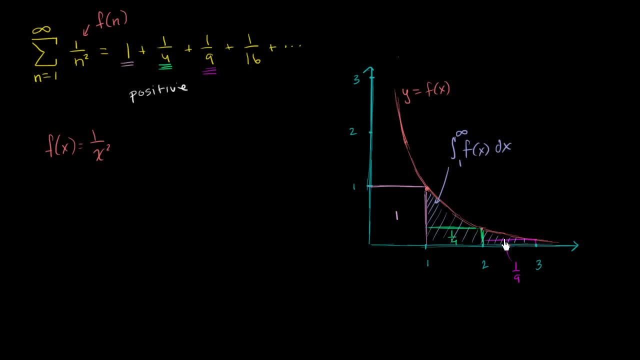 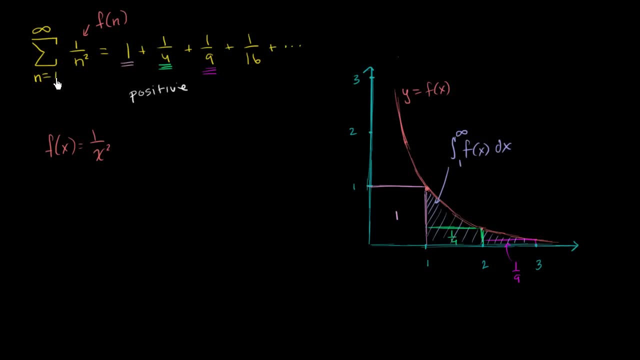 And, as we said earlier, that would be a very good argument for its convergence. So the whole point: here I'm not doing a rigorous proof, but really getting you the underlying conceptual understanding for a very popular test for convergence or divergence, which is called the integral test. 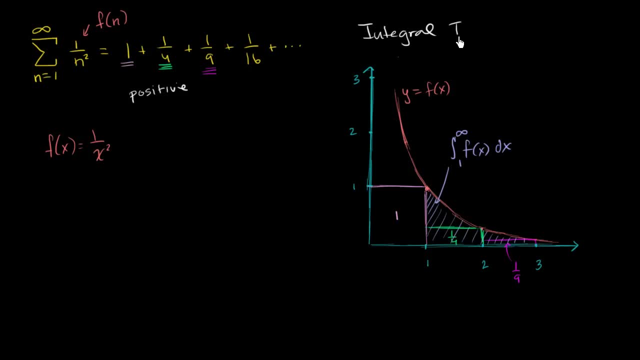 Let me just write that down, just so you know what this is kind of the mental foundations, just so you know what this is kind of the mental foundations, which is kind of the mental foundations, and I'm going to do it in a minute. 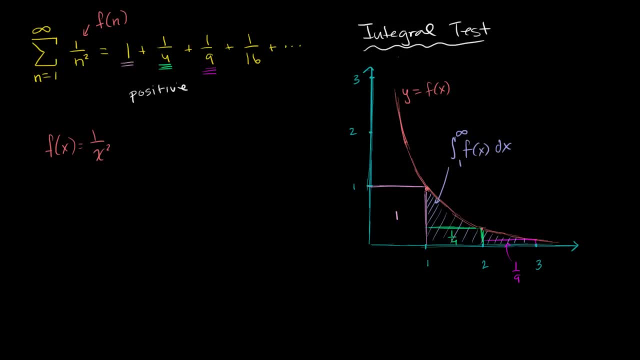 I'm going to do it in a minute. So what do I mean here? So let me write this sum again. Let me write it a little bit different. So our original series from n equals one to infinity of one over n. squared, It's going to be equal to this first block. 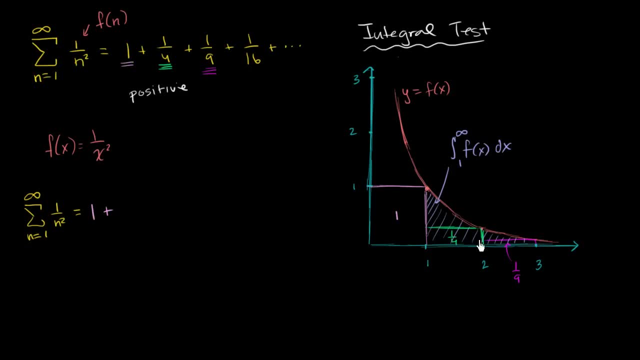 the area of this first block plus the area of all of the rest of the blocks, the one fourth plus one ninth plus one 16th, which we could write, which we could write as the- let me do this in a new color. 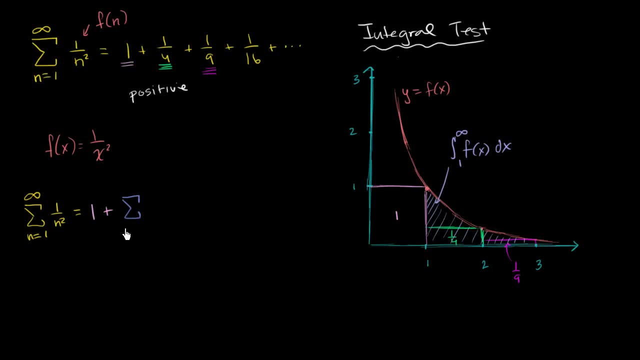 which we could write as: the sum from n equals two to infinity, of one over n squared. So I just kind of express this as the sum of this plus all of that stuff. Now, what's interesting is that this, this, what I just wrote in this blue notation- 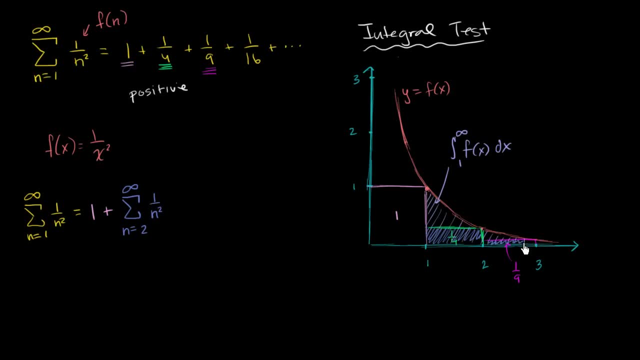 that's this block plus this block, plus the next block, which is going to be less than this definite integral right over here. This definite integral, notice, it's an underestimate. It's always below the curve. So it's going to be less than that definite integral. 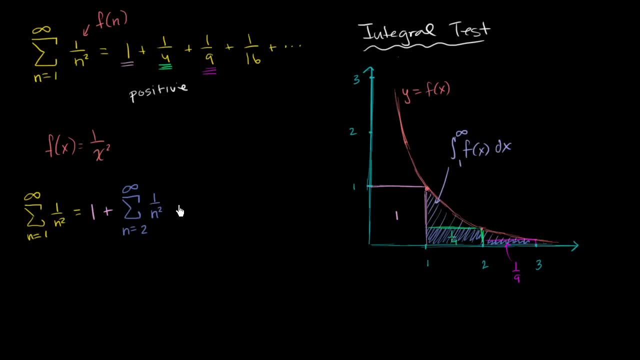 So we can write that this thing is going to be less than one, one plus. instead of writing this, I'm gonna write the definite integral, One plus the definite integral from one to infinity of one over one over x squared dx. 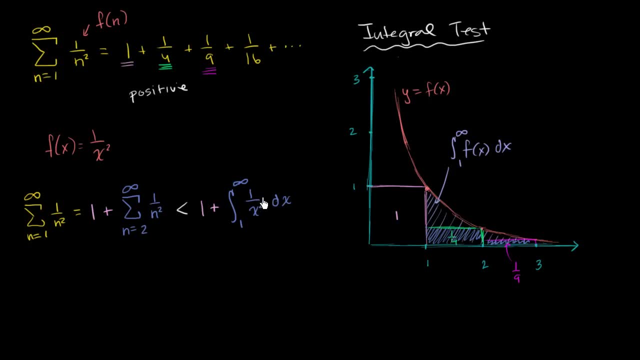 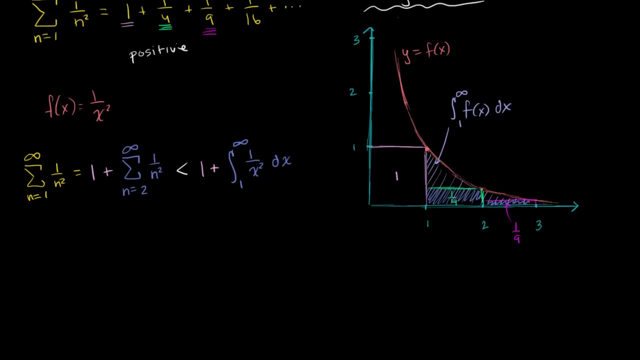 Now, why is that useful? Well, we know how to evaluate this. I encourage you to review the section on Khan Academy on improper integrals if this looks unfamiliar, But I'll evaluate this. I'll evaluate this down here. We know that this is the same thing as the limit. 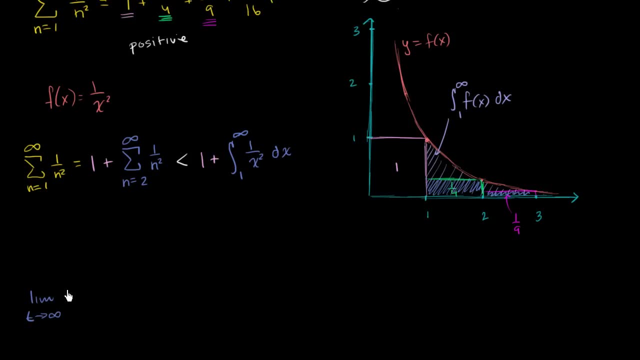 as I'm gonna introduce a variable here. t approaches infinity of the definite integral, from one to t, of, and I'll just write this as: x to the negative, two dx, which is equal to the limit as t approaches infinity of. let's see the of negative x to the negative one. 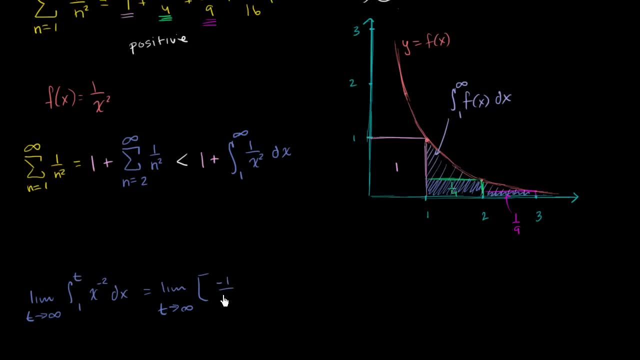 or actually I could write that as negative one over x, negative one over x, and we're gonna evaluate that as t and at one which is equal to the limit, as t approaches infinity, of negative one over t, and then minus, negative one over one.